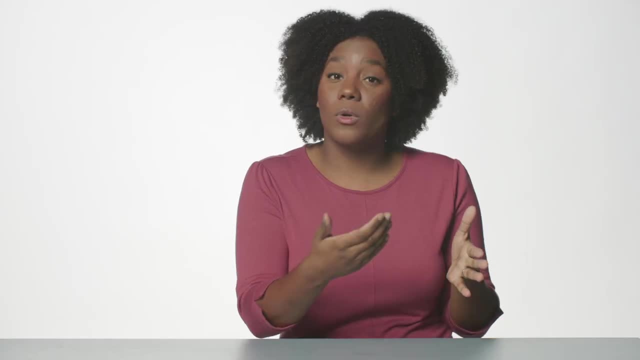 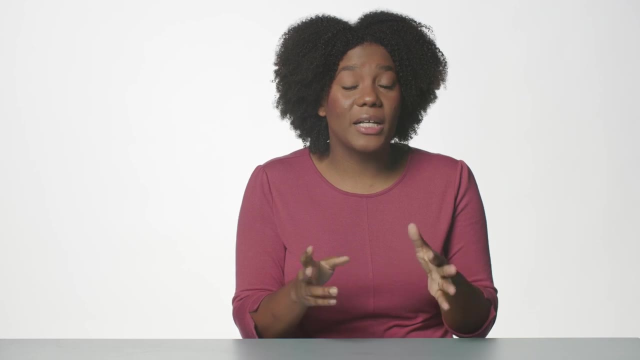 heat transfers between the warm mold and the cold air inside the freezer. The heat from the mold and juice transfers until no energy is available in the juice for the whole time. When the liquid and juice are combined, the heat from the mold and the juice are transferred into the cold air When the 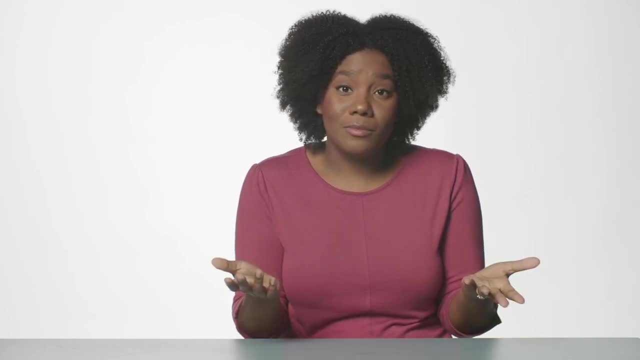 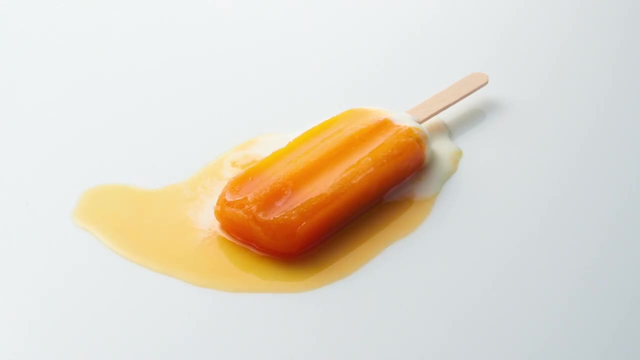 cold air is combined. the heat is transferred between the cold air and the cold air When the for the molecules to slide past one another so they stay in place as a solid frozen treat. Once the frozen treat is taken out of the freezer, it will slowly. 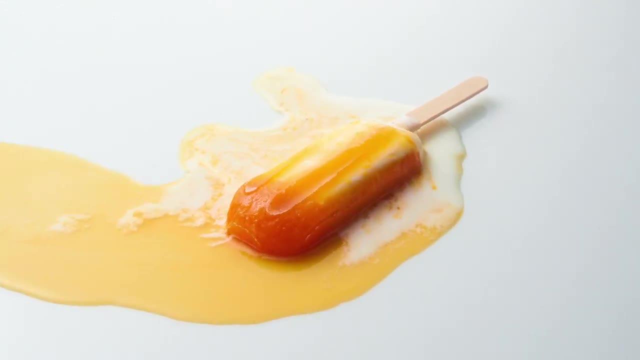 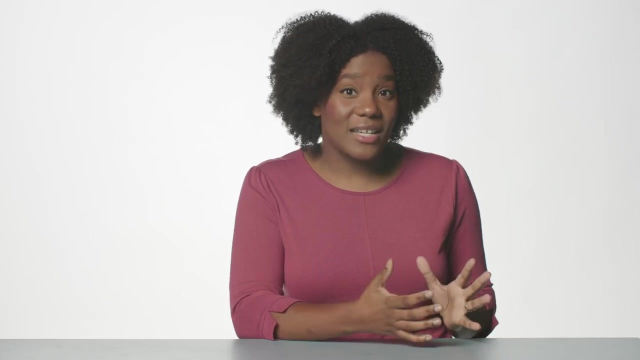 turn back into a liquid as it melts. Since the temperature is much warmer outside the freezer than inside, the solid treat absorbs the surrounding heat, which gives more kinetic energy to the molecules, so they are free to move around. again, The frozen treat changes phases and becomes a liquid. 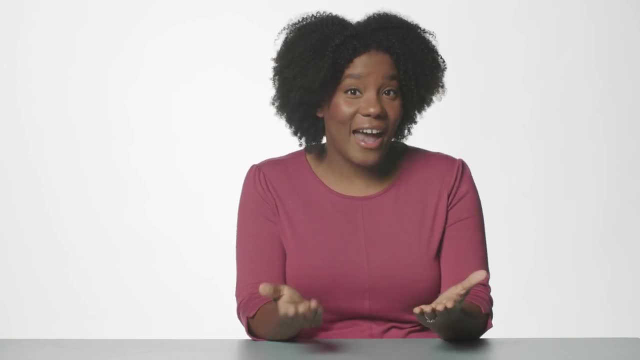 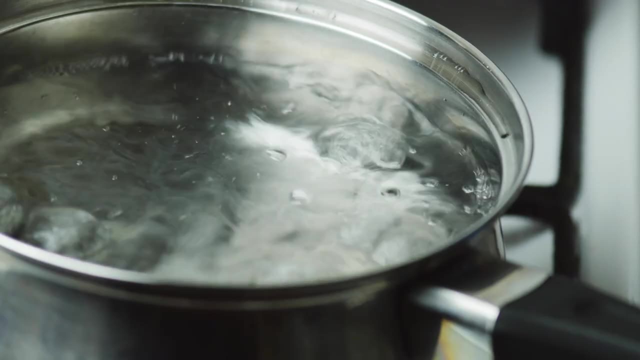 Next, let's look at the changes between liquids and gasses. If you fill a pot with cold water and place it on a hot stovetop, the water heats up. Heat energy travels from the stovetop to the pot and the water absorbs the energy. 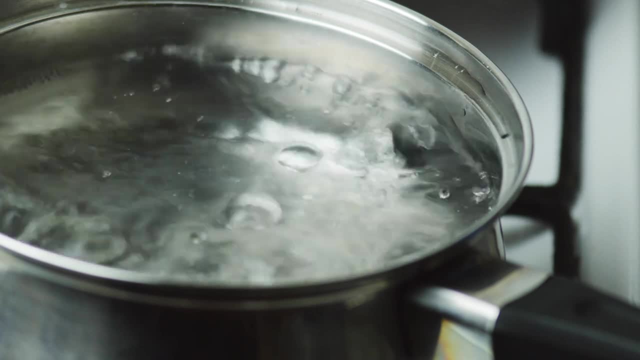 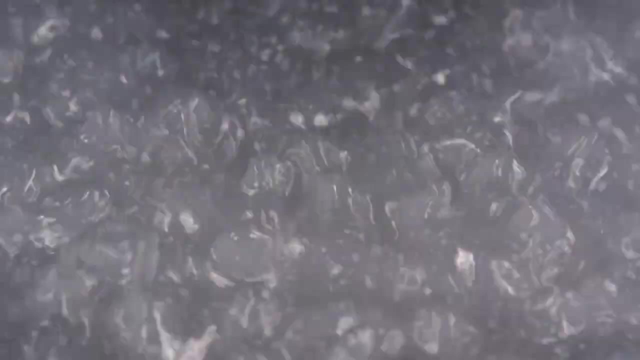 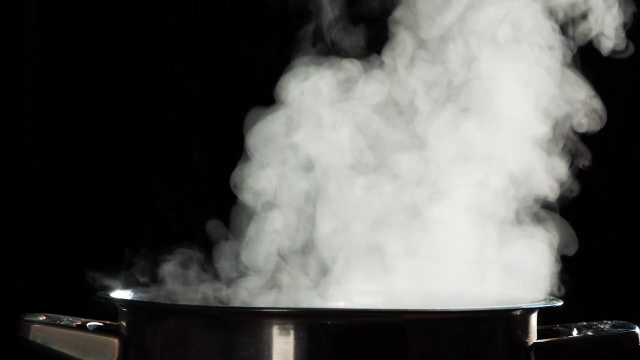 from the pot. Once the water is hot enough, it will start to boil, forming bubbles of water vapor in the pot of water. These bubbles are created as particles of liquid water gain enough kinetic energy to move freely and change to gas. The bubbles rise through the water and leave the pot as steam. 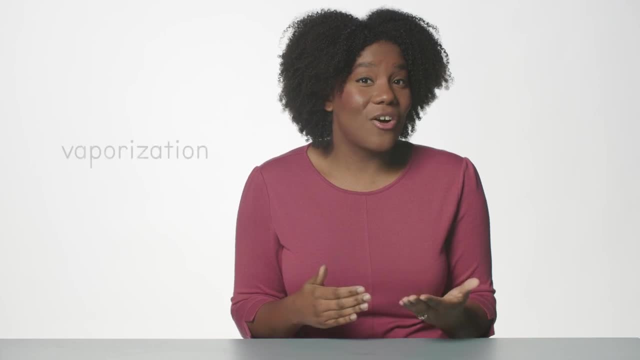 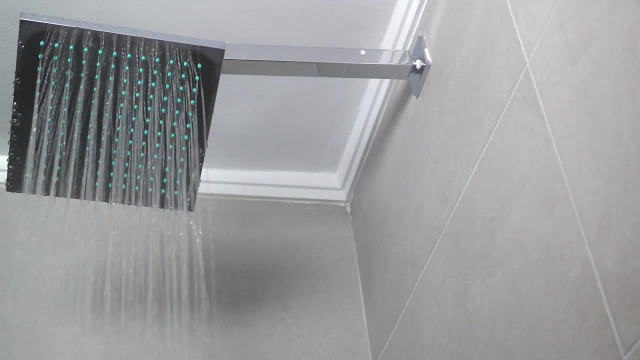 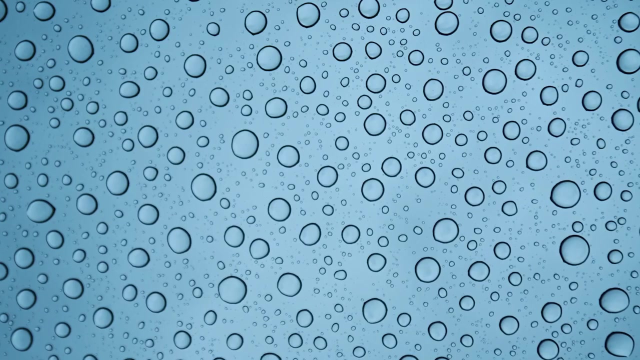 The process in which a liquid boils and changes to a gas is called vaporization. Have you ever noticed that if you take a shower, the bathroom mirror fogs up? This happens because some of the hot water from the shower evaporates. When the hot water touches the mirror, which is cooler, it loses kinetic energy. 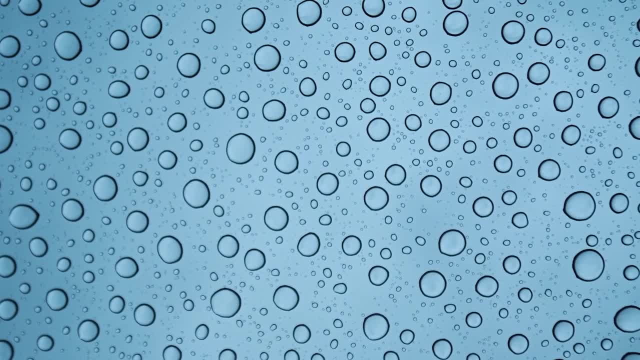 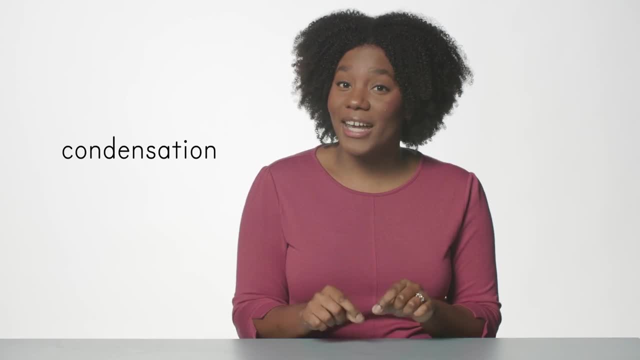 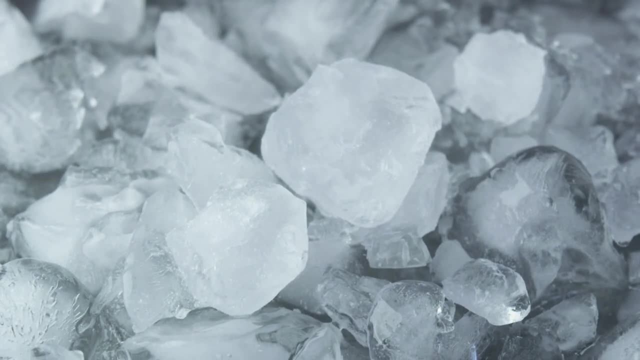 These water droplets now come together and form liquid droplets on the mirror. This process is called condensation. The last phase change we will discuss today is the change between solids and gases. Generally, solids that change to gas will pass through the liquid state first, but sometimes 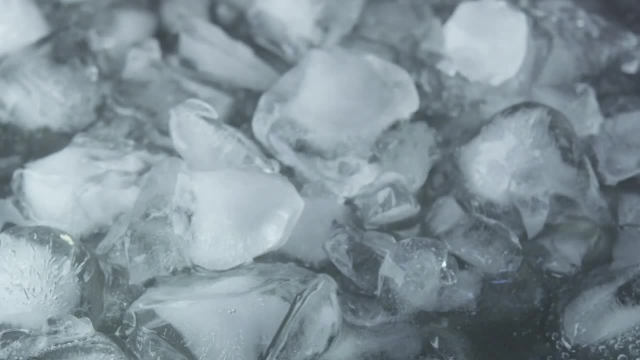 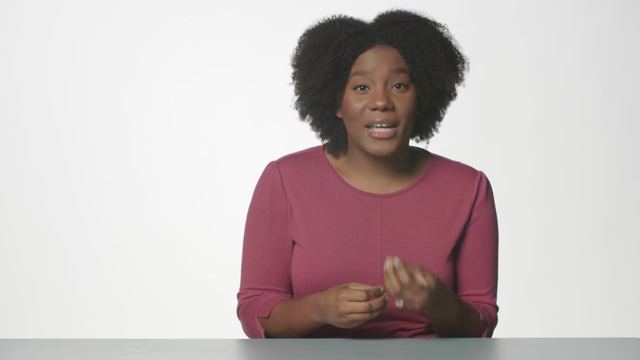 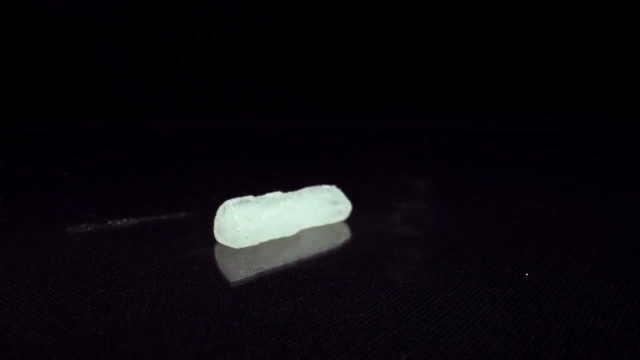 solids skip a state and change directly to gas. The opposite can also happen where gases change directly into solids. When a solid changes directly into a gas, it is called sublimation. Let's watch this process happen with this dry ice. Dry ice is the solid frozen form of the gas carbon dioxide.